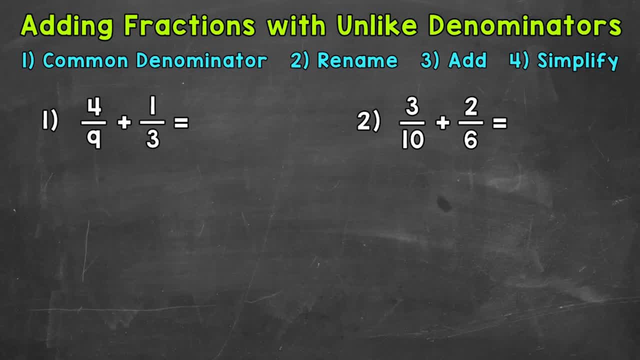 Right away when you see the problem, but if not, you can always write out your lists of multiples in order to find it. Let's write out the multiples of nine and three, So I'll come to the bottom of the screen where I have some extra room to write out these lists. We'll start with. 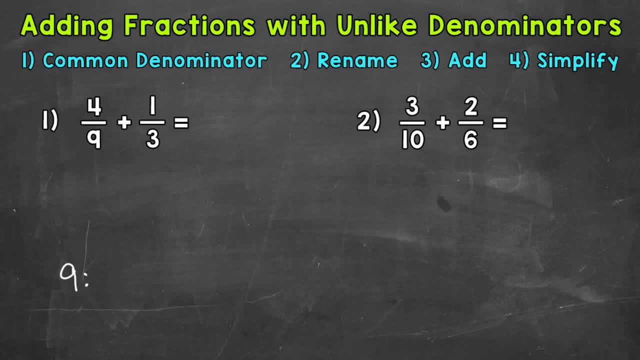 nine, So nine. the first multiples of nine are nine, eighteen, twenty-seven, thirty-six, So I'll write four multiples of nine there. I would suggest writing out four or five multiples of each. See if you have any common multiples, and if not, you can always extend your lists. So let's. 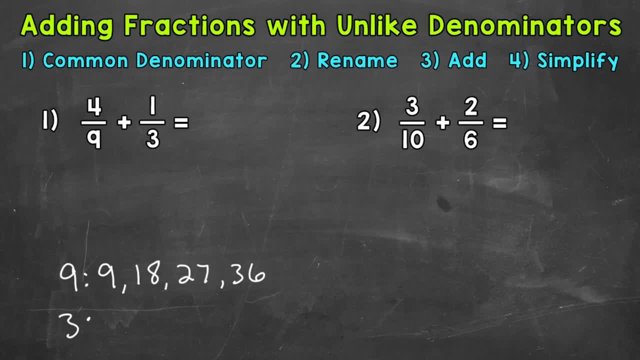 do three now and see if we have any common multiples. Three, six, nine, and it looks like we have a common multiple of nine And, more specifically, that's going to be the least common multiple of nine. So let's do three now and see if we have any common multiples of nine. 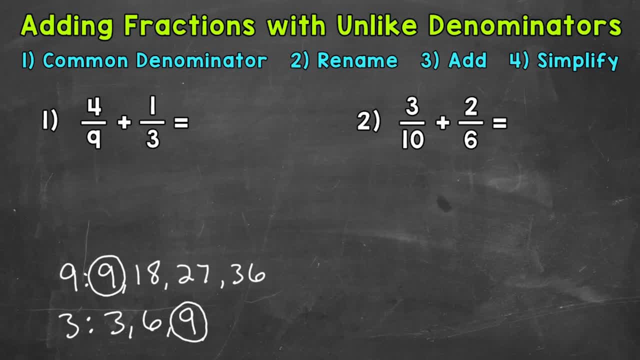 We always want to find the least common multiple. Smaller numbers in value are generally easier to work with and this will help cut down on simplifying in the end. So nine is going to be our common denominator. Let's come back up to the original problem and rename these fractions with: 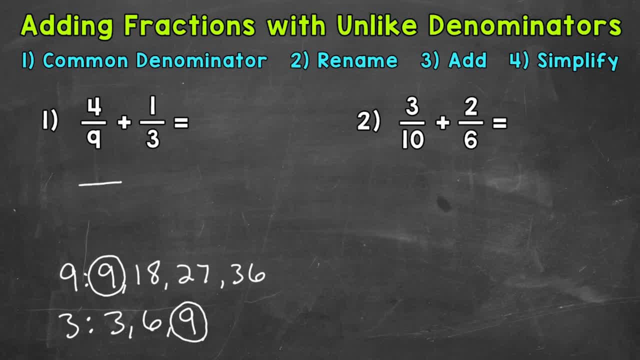 our common denominator of nine. So underneath I'm going to write our common denominator of nine and now we can rename. So we'll start with four-ninths. Well, four-ninths already has a denominator of nine, so we don't need to rename. So we can just bring the four down. As far as 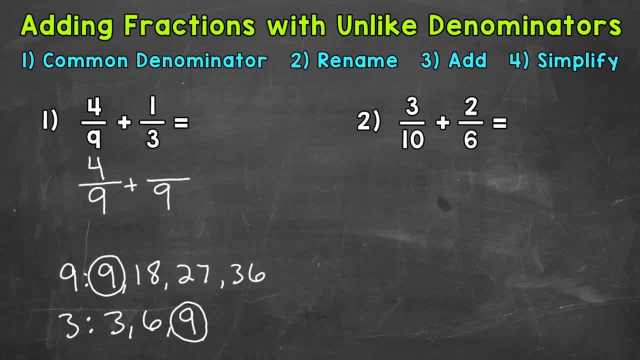 one-third, we need to think: three times what equals nine. How do we get three to equal nine? Well, we know, three times three equals nine. Now, in order to rename, we want to first have an equivalent fraction. We want to keep this equivalent. We do not want to change. 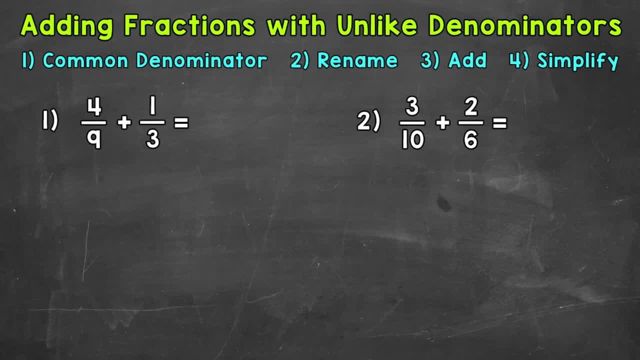 Right away when you see the problem, but if not, you can always write out your lists of multiples in order to find it. Let's write out the multiples of nine and three. So I'll come to the bottom of the screen where I have some extra room to write out these lists. We'll start with nine. So nine, the first multiples of nine are nine, eighteen, twenty-seven, thirty-six. So I'll write four multiples of nine there. I would suggest writing out four or five multiples of each. See if you have any common multiples, and if not, you can always extend your lists. So let's do three now and see if we have any common multiples. Three, six, nine, and it looks like we have a common multiple of nine. And more specifically, that's going to be the least common multiple of nine. So let's do three now and see if we have any common multiples of nine. 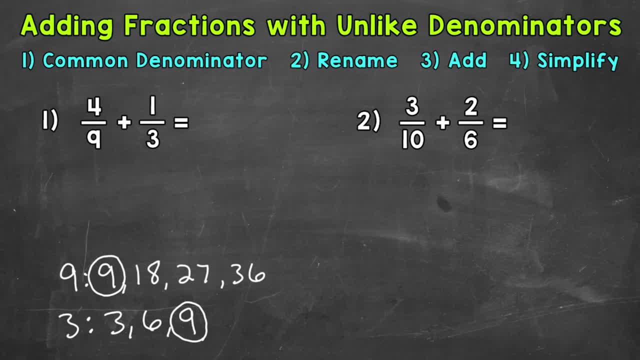 We always want to find the least common multiple. Smaller numbers in value are generally easier to work with, and this will help cut down on simplifying in the end. So nine is going to be 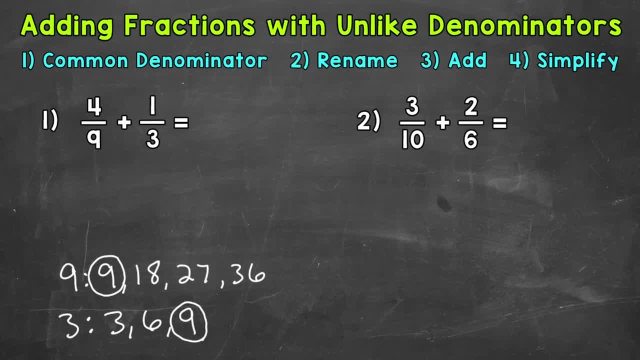 our common denominator. Let's come back up to the original problem and rename these fractions with our common denominator of nine. So underneath, I'm going to write our common denominator of nine, 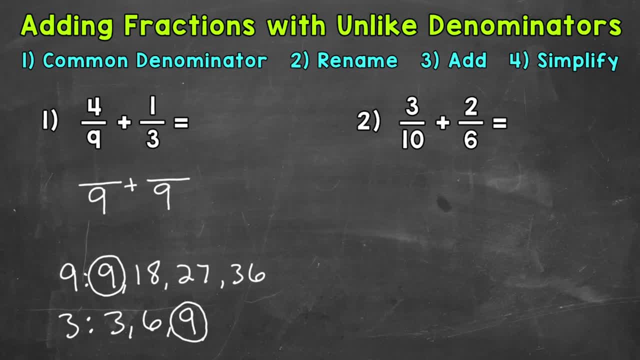 and now we can rename. So we'll start with four-ninths. Well, four-ninths already has a denominator of nine, so we don't need to rename. So we can just bring the four down. As far as 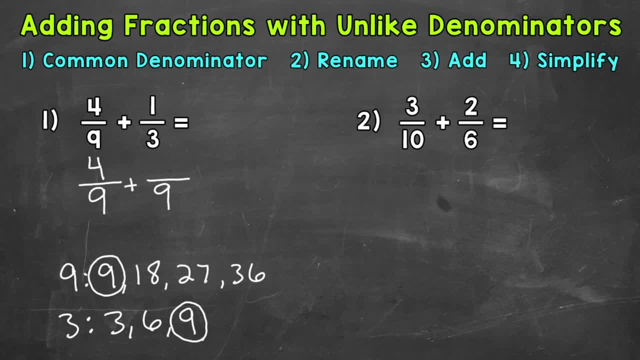 one-third, we need to think three times what equals nine? How do we get three to equal nine? Well, we know three times three equals nine. Now, in order to rename, we want to, 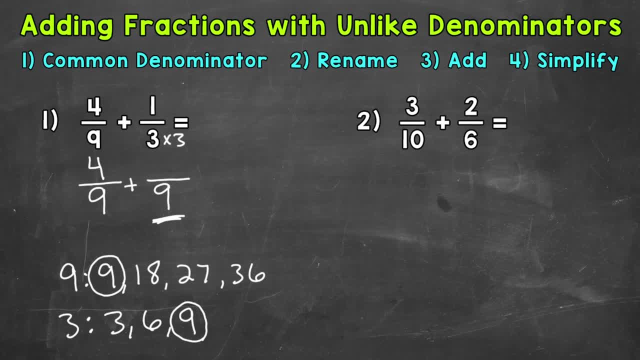 first, have an equivalent fraction. We want to keep this equivalent. We do not want to change the value of the problem at all. So whatever we do to the denominator, we have to do to the numerator. So one times three is three. Three-ninths is equivalent to one-third, but we have that common 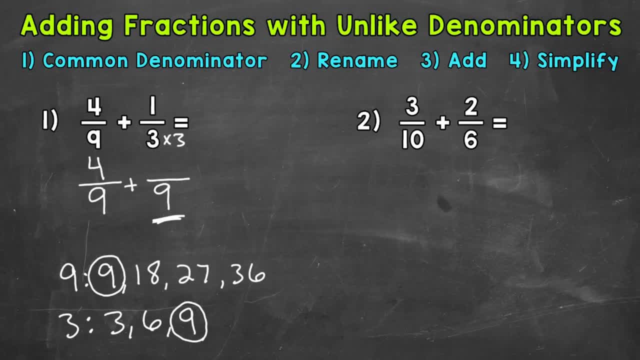 the value of the problem at all. So whatever we do to the denominator, we have to do to the numerator. So one times three is three. Three-ninths is equivalent to one-third, but we have that common denominator of nine. now, Now that both fractions have a common denominator, we can add. So when we 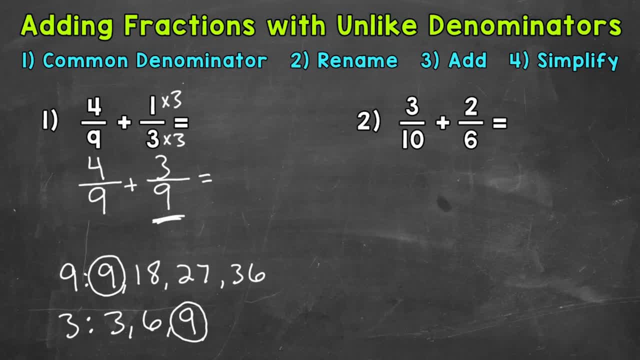 add fractions, we add the numerators, the top numbers. Four plus three is seven, And then we keep the denominator the same, So nine Seven-ninths is our final answer. Now it's common practice to simplify fractional answers, So we look to see if we can break this fraction down at all. 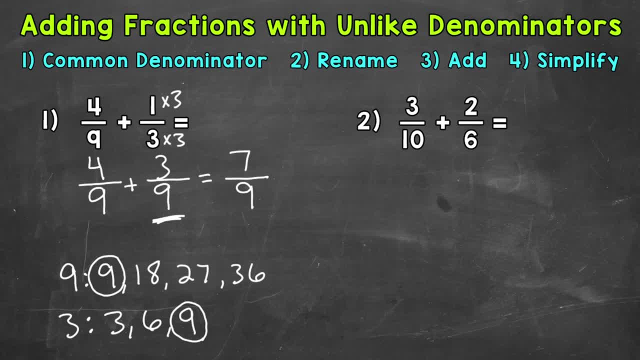 Are there any common factors between seven and nine besides one? Can we simplify? No, The only common factor between seven and nine is one. So this is in simplest form and we are done. Seven-ninths is our final answer. Let's try another one and move on to. 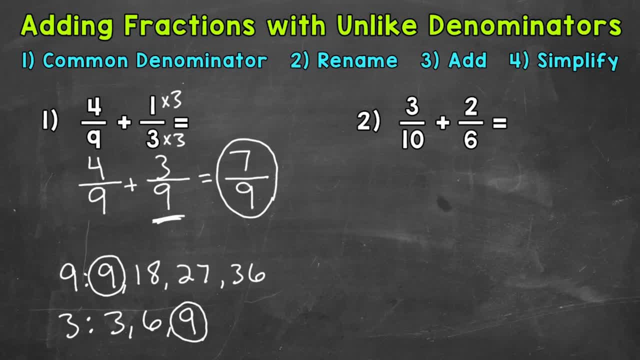 number two, where we have three-tenths plus two-sixths. So the first thing that we want to do, we need to find a common denominator. So let's write out the multiples of ten and six. We'll start with the denominator. So let's write out the multiples of ten and six. 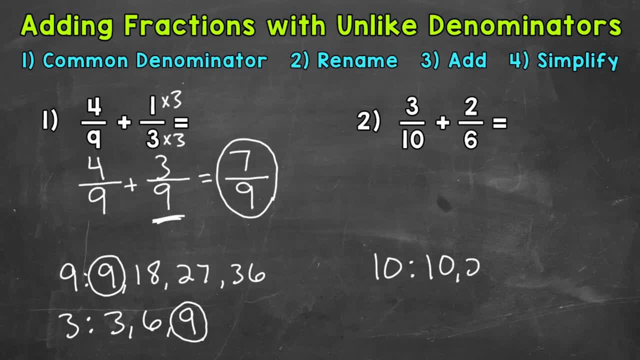 We'll start with ten, So ten, twenty, thirty, forty. So we'll write out four multiples for each. Let's do six now, Six, twelve, eighteen, twenty-four, So four for each, and we don't have a common multiple. That's okay, We can extend our lists. Now the multiples of ten: we're already. 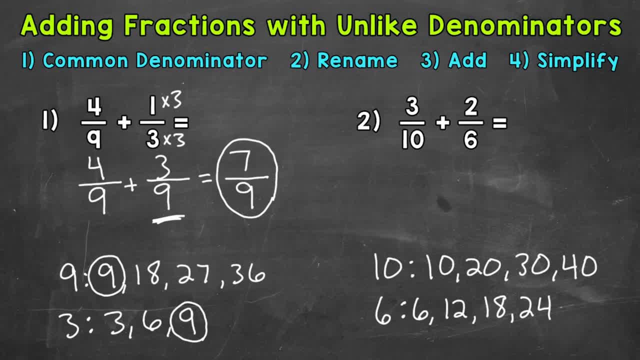 at forty- and the multiples of six. we're already at twenty-four, So we can extend our lists. Six, we're only at twenty-four, so let's extend that list. So after twenty-four would be thirty. and now we have a common multiple and specifically the least common multiple. 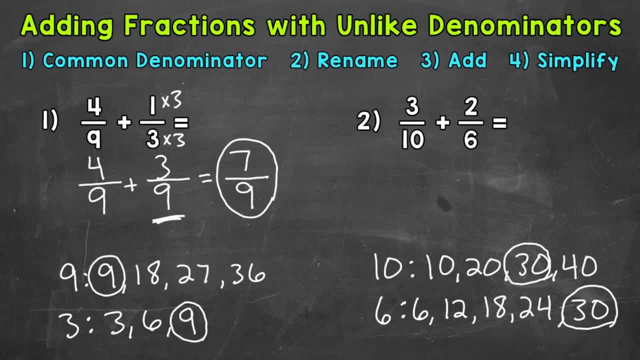 So thirty is going to be our common denominator. Let's rename our fractions with that denominator of thirty, Let's start with three-tenths. So we need to think in order to keep this equivalent. whatever we do to the denominator, we have to do to the 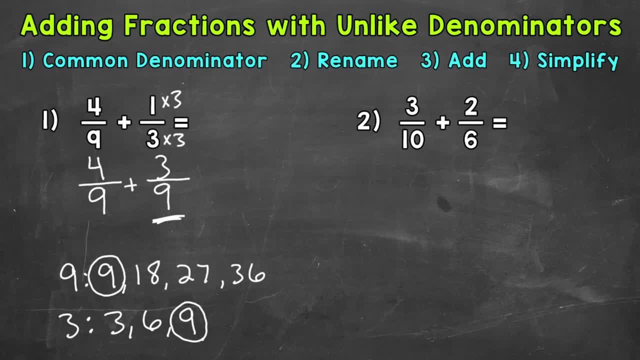 denominator of nine now. Now that both fractions have a common denominator, we can add. So when we add fractions, we add the numerators, the top numbers. Four plus three is seven. And then we keep the denominator the same. So nine. Seven-ninths is our final answer. Now, it's common practice 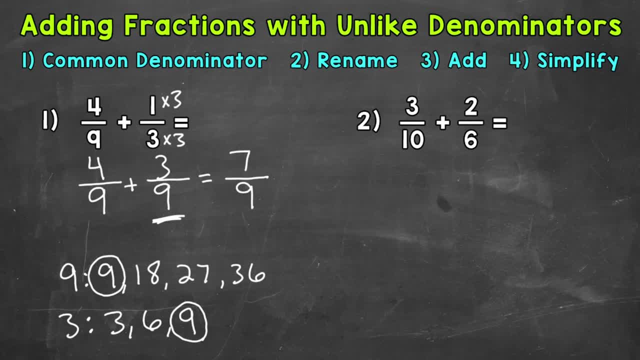 to simplify fractional answers. So we look to see if we can break this fraction down at all. 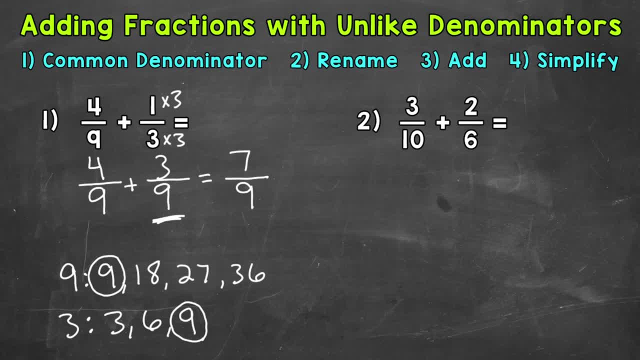 Are there any common factors between seven and nine besides one? Can we simplify? No. The only common factor between seven and nine is one. So this is in simplest form, and we are done. Seven-ninths is our final answer. Let's try another one and move on to 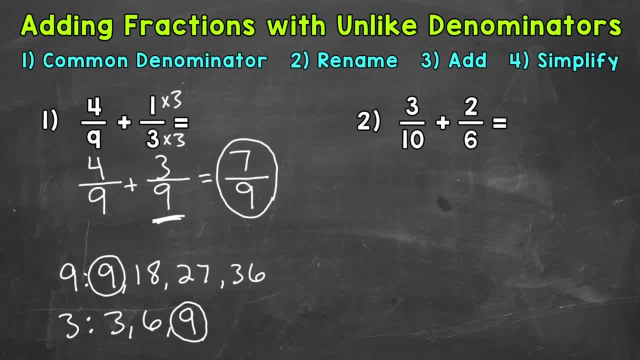 number two, where we have three-tenths plus two-sixths. So the first thing that we want to do, we need to find a common denominator. So let's write out the multiples of ten and six. Okay. We'll start with 10. So 10, 20, 30, 40. So we'll write out four multiples for each. Let's do six now. Six, 12, 18, 24. So four for each, and we don't have a common multiple. That's okay. We can extend our lists. Now, the multiples of 10, we're already at 40, and the multiples of six, we're only at 24. So let's extend that list. So after 24 would be 30, and now we have a common multiple, 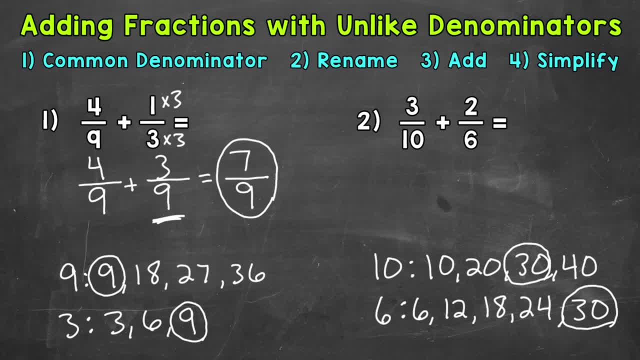 and specifically, the least common multiple. So 30 is going to be our common denominator. 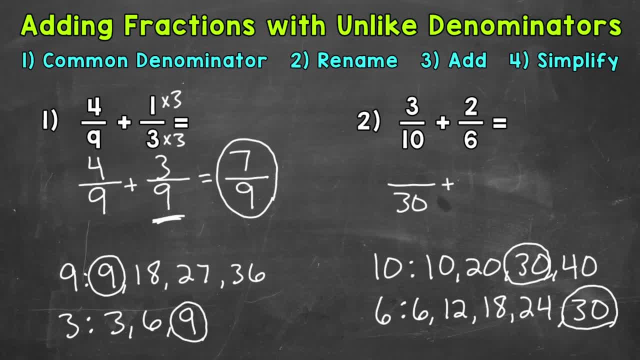 Let's rename our fractions with that denominator of 30. Let's start with three-tenths. So we need to think, how do we get 10 to equal 30? 10 times what equals 30? Well, 10 times 3 equals 30. We know 10 times 3 equals 30. In order to keep this equivalent, whatever we do to the denominator, we have to do to the numerator. So multiply the numerator by 3 as well. 3 times 3 is 9. So 9-thirtieths is equivalent to 3-tenths, but we have that common denominator of 30 now. 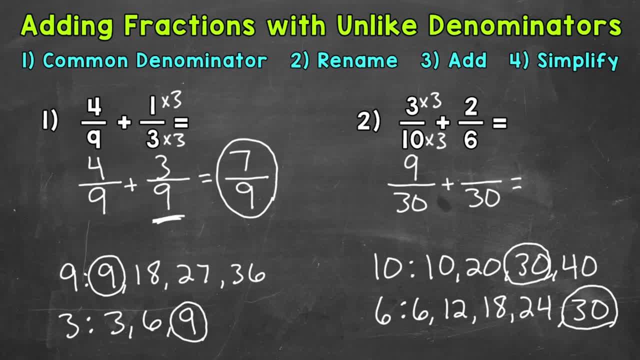 We do 2-sixths. So we think, how do we get 6 to equal 30? 6 times what is 30? Well, 6 times 5 is 30. Whatever we do to the denominator, we do to the numerator. So 2 times 5 gives us 10. 10-thirtieths is equivalent to 2-sixths. Now that we found the common denominator, we renamed. We can add. So add the numerators. 9 plus 10. 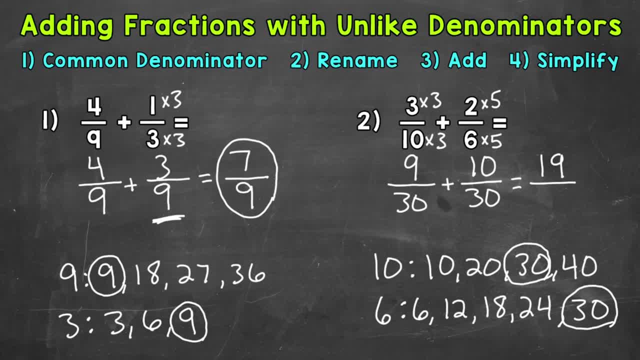 Is 19. Keep the denominator of 30. And our final answer is 19-thirtieths. We can check to see if we 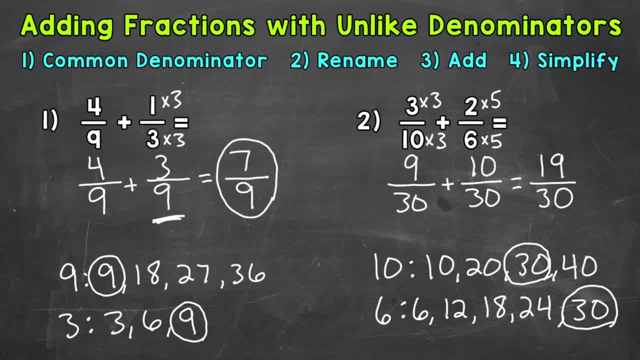 can simplify, but 19-thirtieths is in simplest form. The only common factor between 19 and 30 is 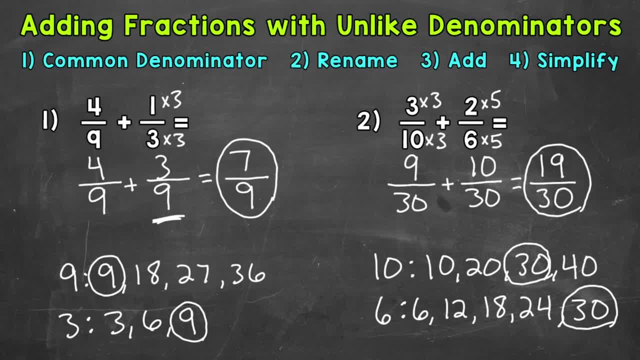 1. So we are done. So there you have it. There's how you add fractions with unlike denominators. 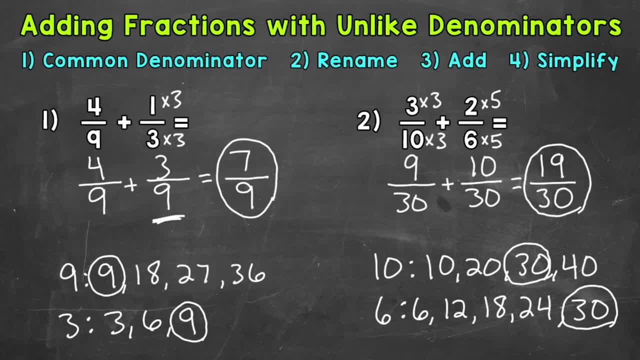 Find a common denominator. Rename with that common denominator. Add. And then look to see if you can simplify. Now there is a part 2. I'll add that link down in the description. 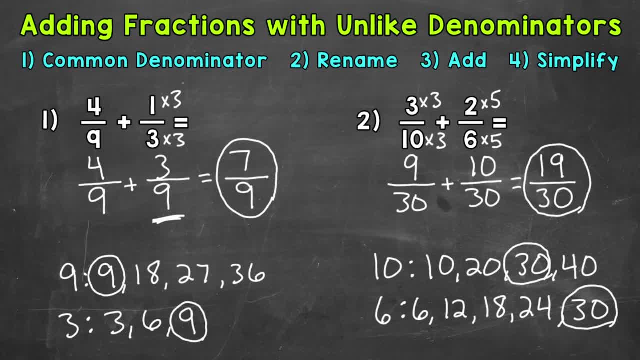 Part 2 will have two more examples. And in one of those examples, there's an answer that can be simplified. 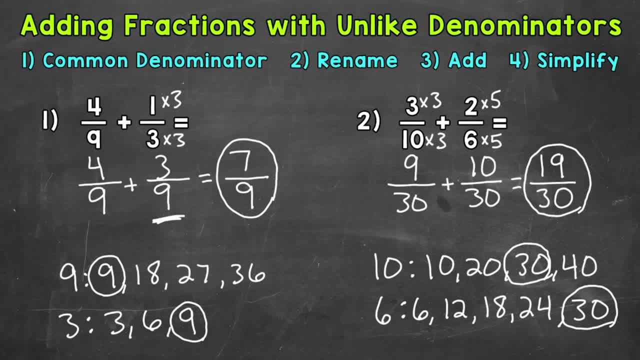 So you can see what that looks like. Also, if you need more help with multiples and least common multiple, I'll have a link to that video in the description as well. I hope that helped. Thanks so much for watching. Until next time. Bye. Until next time. Peace. 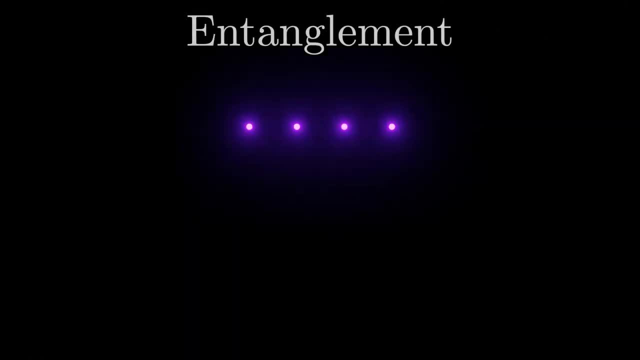 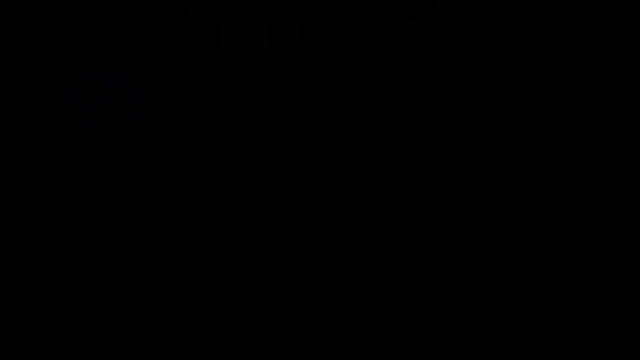 Entanglement is a strange property of multiple qubits that allows them to carry more information than the individual qubits carry by themselves. For example, if we pass two qubits through this specific set of gates, then measure them afterwards. we find that we always measure. 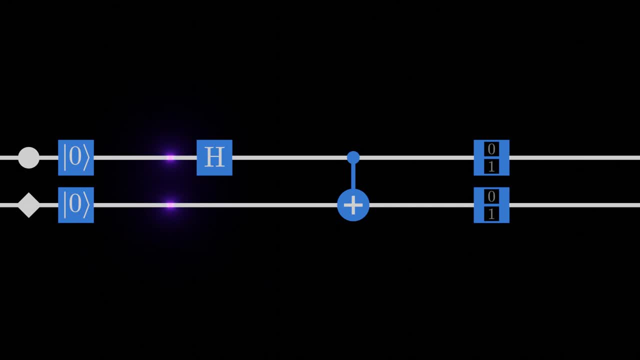 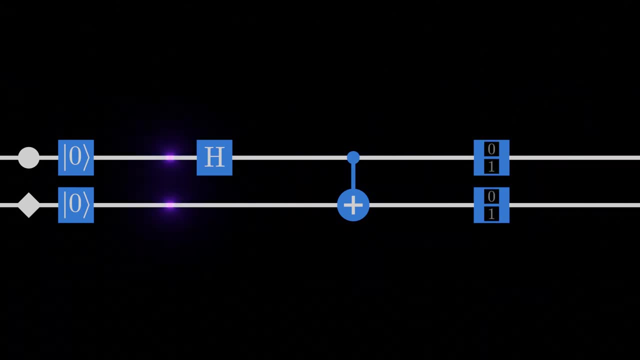 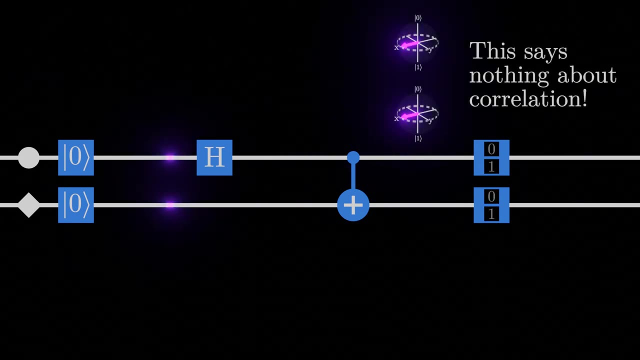 them as both zero or both one. This ability for multiple measurements to be correlated is an essential property of entanglement. It tells us that the behavior of qubits together can't be explained by describing each qubit individually. To start, we'll represent a system.